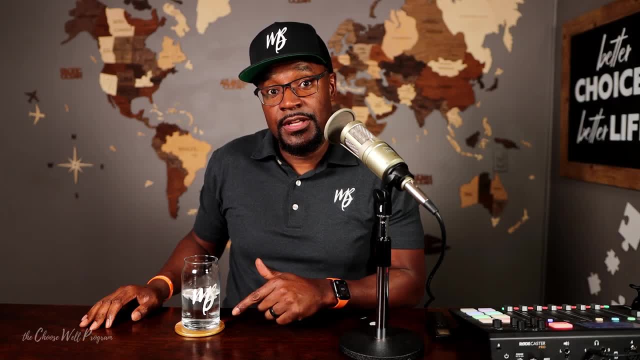 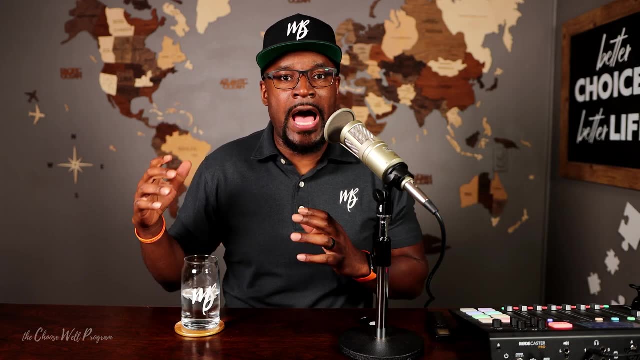 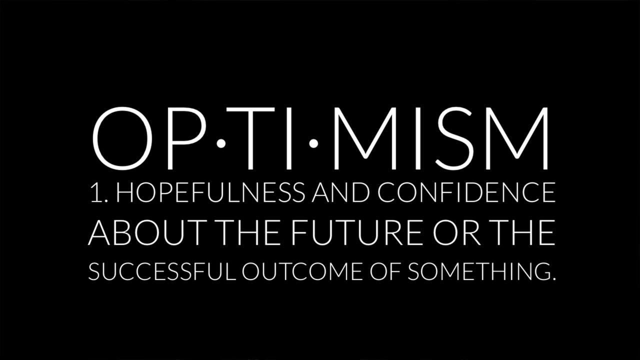 It's half empty or it's half full. How do you see this glass? All depends on your perspective. How do you see things? Today, I want to talk about this idea of optimism. Optimism is the hopefulness and confidence about the future or the successful outcome of something. In other words, 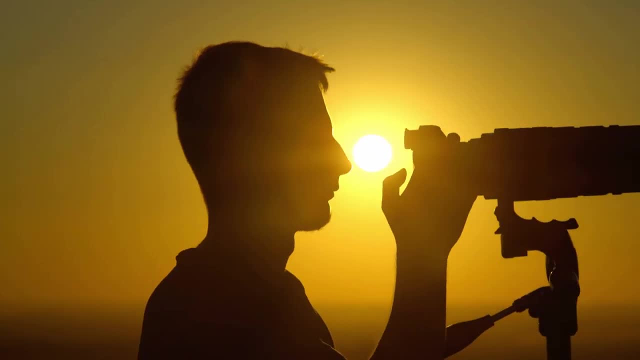 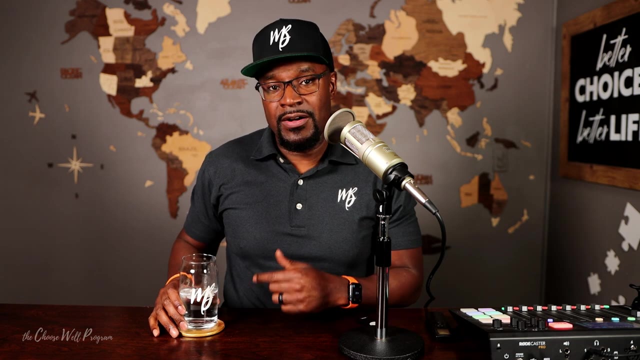 optimism is looking on the bright side of things. You look at this glass. an optimist or a person looking with optimism would say this glass is half full, while a pessimist would say this glass is half empty. I don't think you have to be either an optimist or a pessimist, but I think it's. 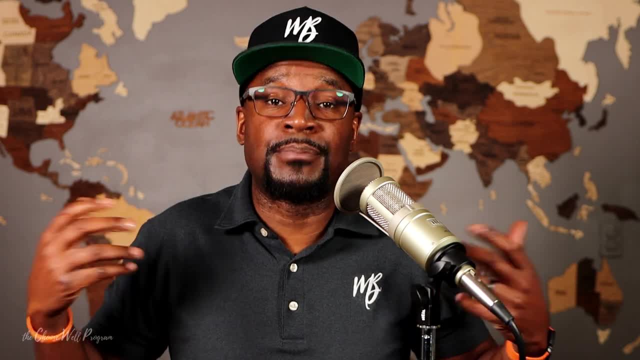 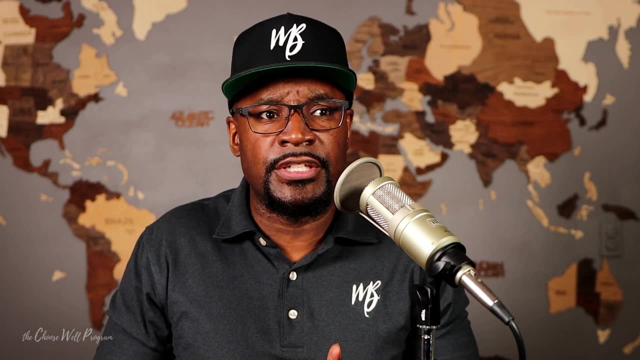 important to always Focus on trying to look at the bright side of things, or I like to say to look for the good. And I try to do that in my own life: to look for the good Now. when I grew up, they would say statements like this: If life gives you lemons, make lemonade. Well, I would say, make. 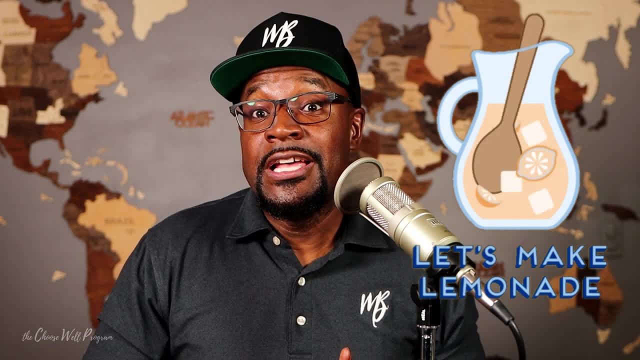 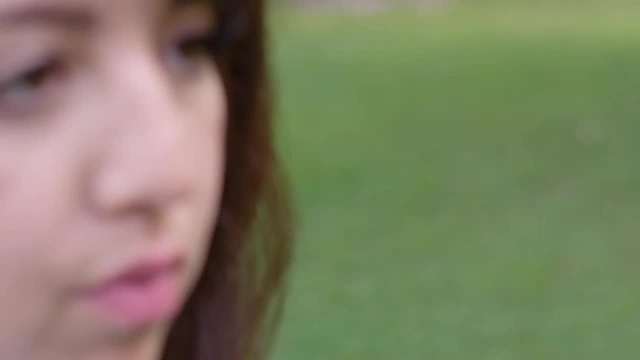 a lemonade smoothie, make a frosty, take whatever you have and do the best with it. See, it doesn't do us any good to look at everything with negativity. Now, I'm not a person who wants to be deceived or be naive to think that I'm a good person. I'm not a person who wants to be. 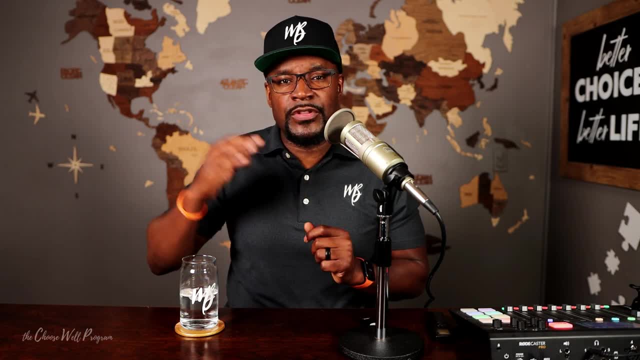 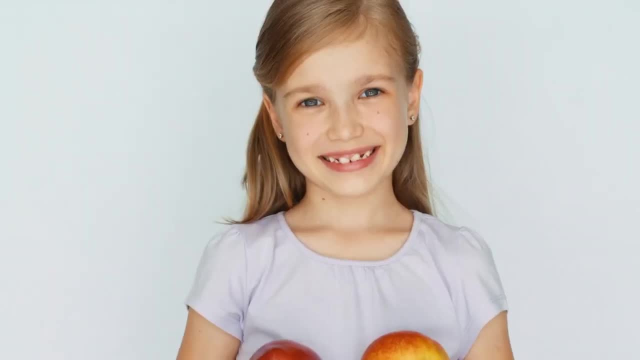 deceived or be naive to think that everything's going to work out perfectly. But I think I can always look for the good side of things. Optimism changes your view on the world. It changes your outcome. I believe when you look at the world with optimism, it helps you be healthy- healthier. 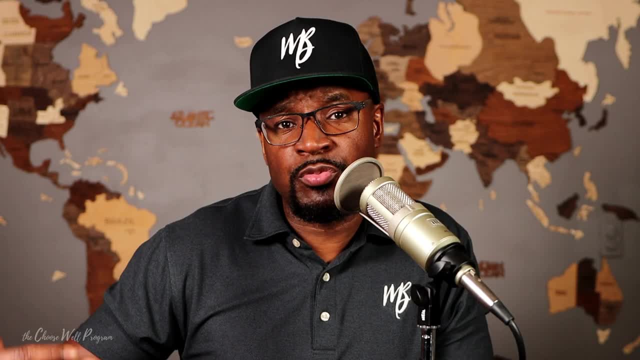 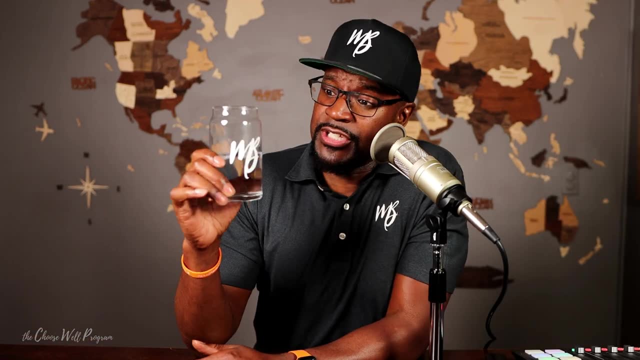 and happy. Yes, things will go wrong, but you can always work to make them better. Yes, this glass is half empty, but you know what? There's still a whole lot of water in here, And if a brother's thirsty, this could come in real handy. 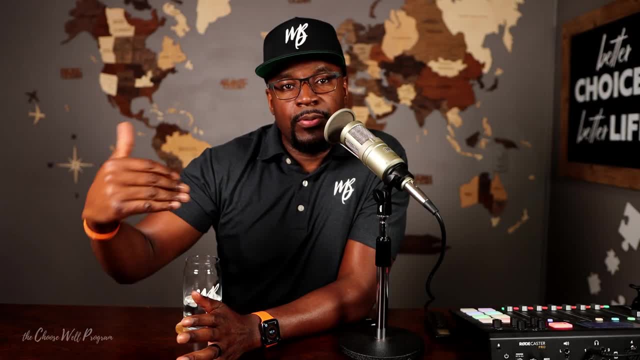 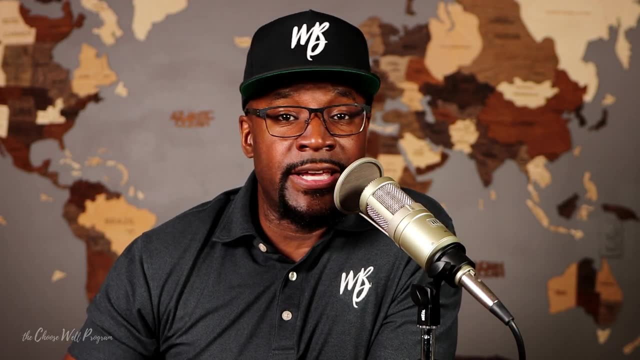 Oh yeah, And sometimes looking for the good can help you progress in life, or or make some progress. For an example, we just had a pandemic over the last 2020 and it caused me to lose a lot of money. I didn't get to go to schools and speak, And so I could sit around and mope about that, But 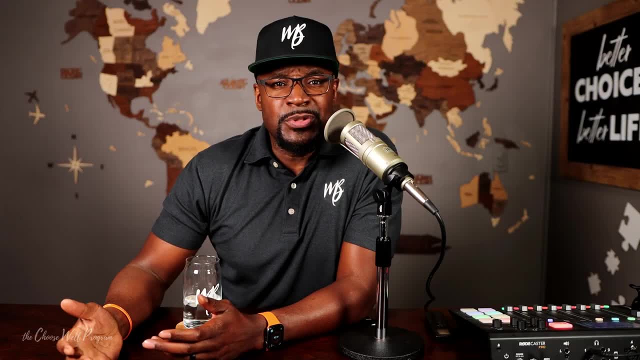 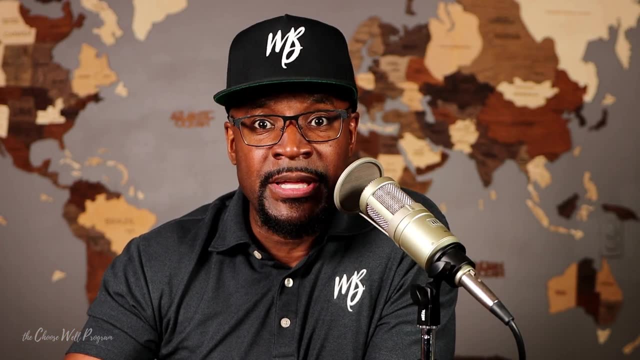 man, I'm never going to get, never going to be able to do anything. Instead of doing that, I look for other ways. I did some virtual things. I made a whole lot of videos. Matter of fact, we made 100 video series during that time, And now those videos are being used across the country and